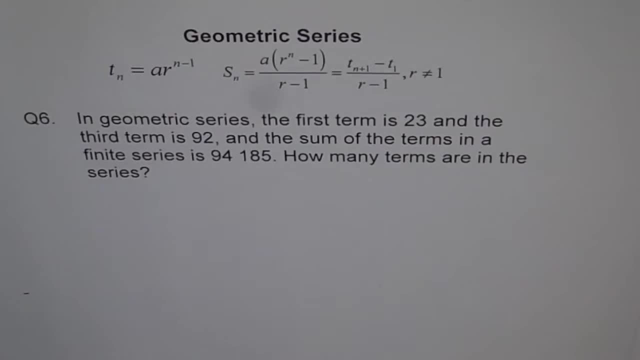 Question 6.. In geometric series, the first term is 23 and the third term is 92. And the sum of the terms in a finite series is 94, 185.. How many terms are in the series? Well, so in geometric series we can write the terms as: Tn equals to a, r to the power of n minus 1,. 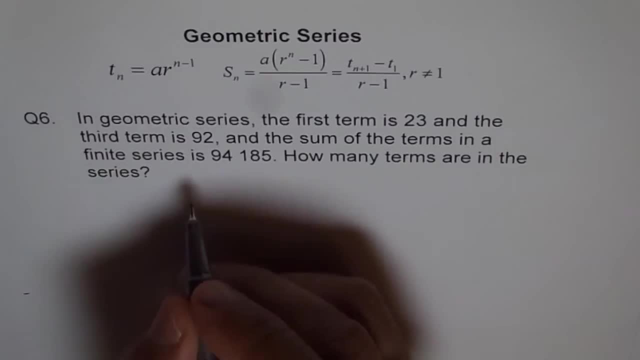 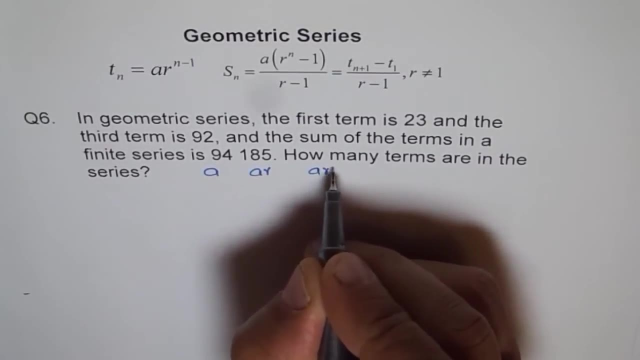 right. So basically the terms are: if the first term is a, the second term is a times r right, Then the third is a times r squared, and then we have a times r cubed like this right Now. 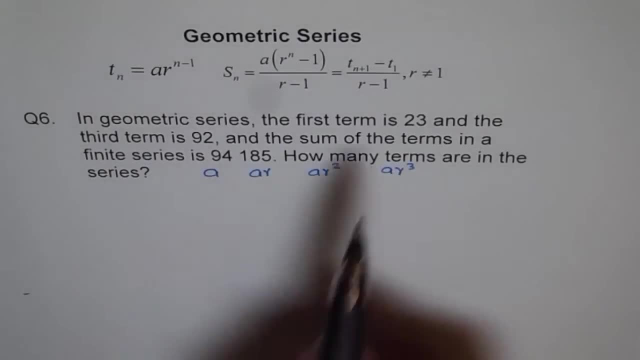 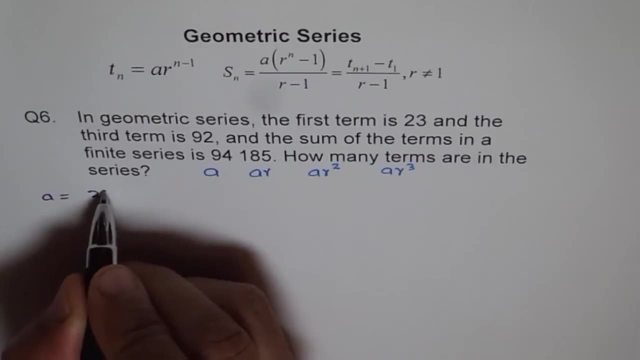 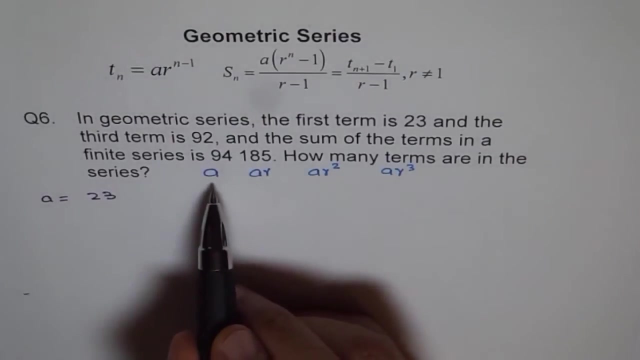 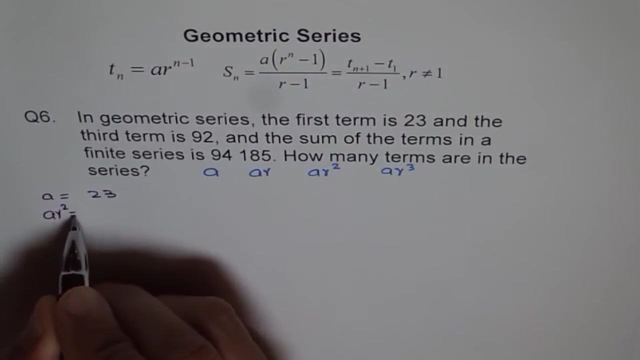 so we have: first term has 23.. That means we can write: a is equals to 23,, correct? Third term is 92.. So third term is: this is the first term, second term, third term. Third is a r squared, correct. So we can write a r squared equals to 92,. 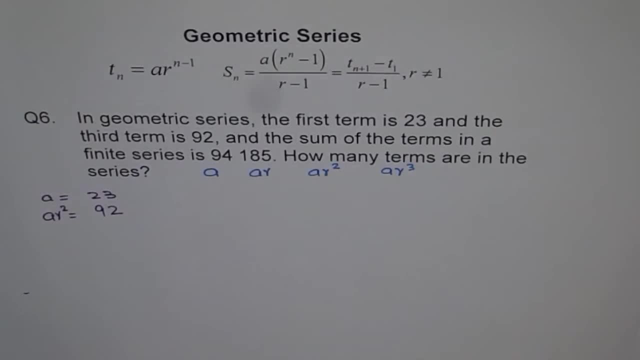 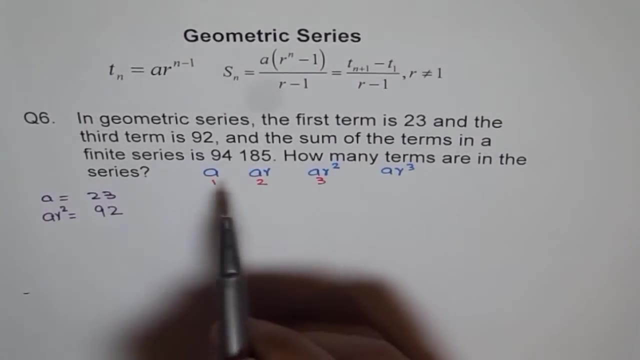 right? These are your terms, right? This is term number 1, this is term number 2, term number 2, this is term number 3, and so on. so first term is a, so a is 23. third term is a r. 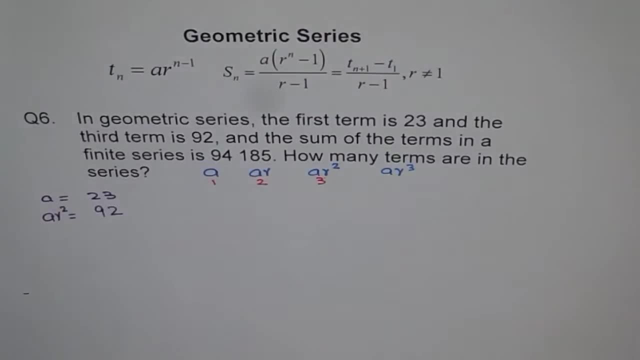 square, which is 92, correct. so we got these two terms now. from here, if i see ratio, if i divide them, if i write a r square divided by a, i've got 92 over 23, correct. so i'll divide one by this, i'll r square over a is equals to 92 over 23, correct? so from here, a and a cancel and we get r square. 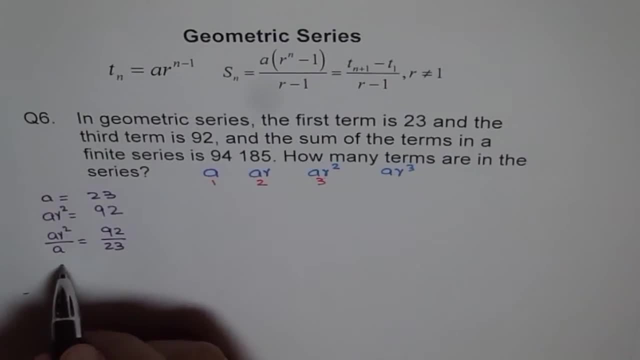 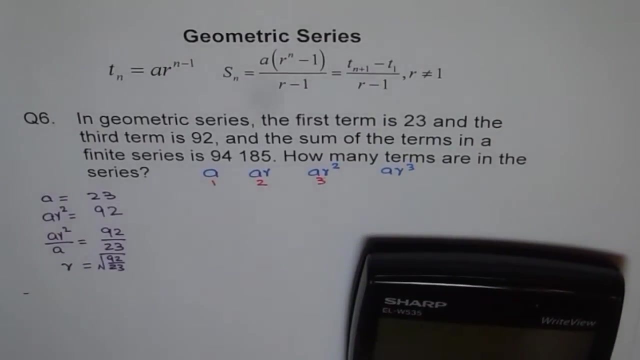 equals to 92 over 23, or r is equals to square root of 92 over 23. let's find out how much is this, so we will do square root of, so we'll divide away from here. let's find out how much is this, so we will do square root of, so we'll divide out. 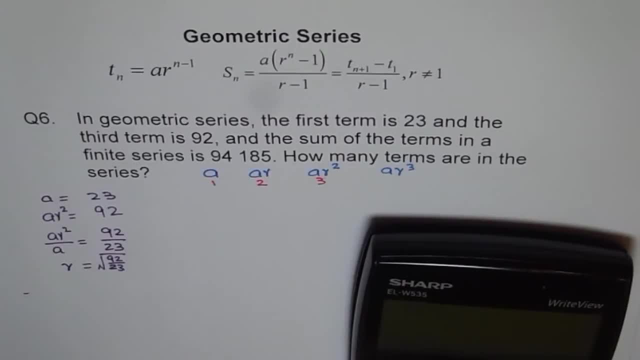 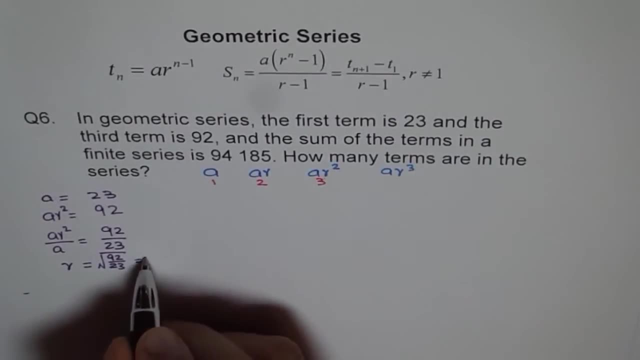 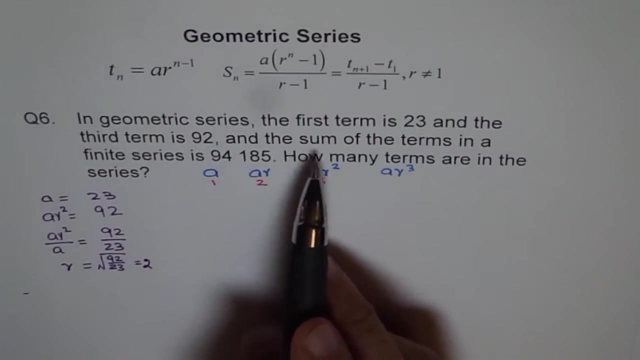 92 by 23,, we get 4, and square root of 4 is 2, right, So we get r equals to 2.. Do you see that? So we get r like this. Now, the sum of the terms in a finite series is this: 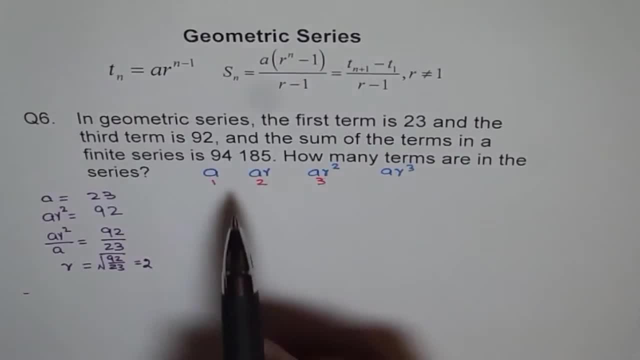 So you know r. now you know a and you know the sum. right. You need to find how many terms are in the series. So you need to find n. So this is a good formula to use this time, correct. Now we know a couple of things. So we know a, we know a. equals to 23,, correct? 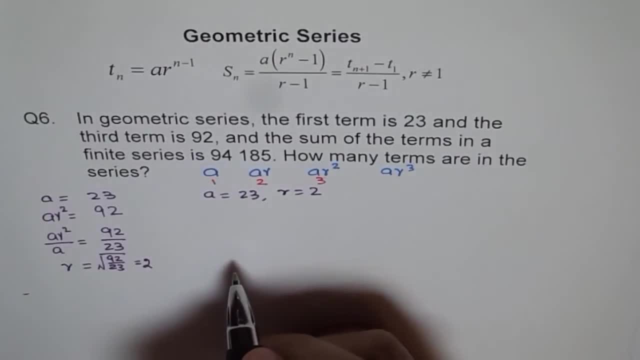 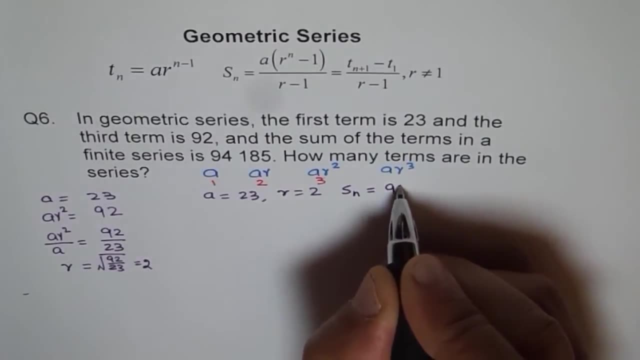 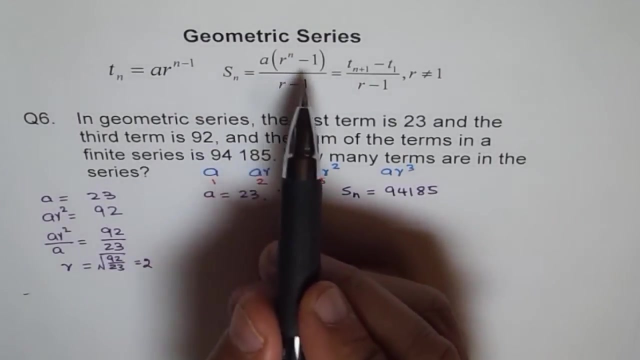 r equals to 2.. And how many terms we want. but we know s of n. So we have s of n equals to 94, 185.. We know all these things. So we know s of n, We know a and we know r. So only variable left is n, which we can find correct. So. 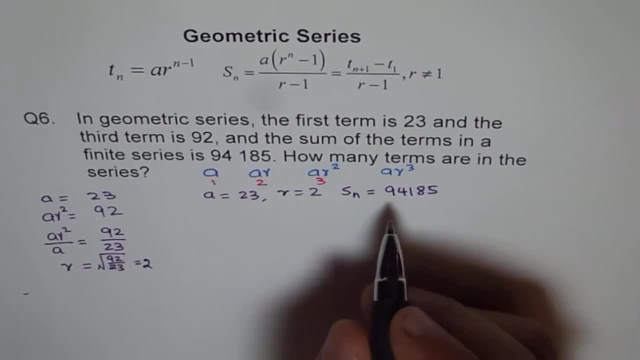 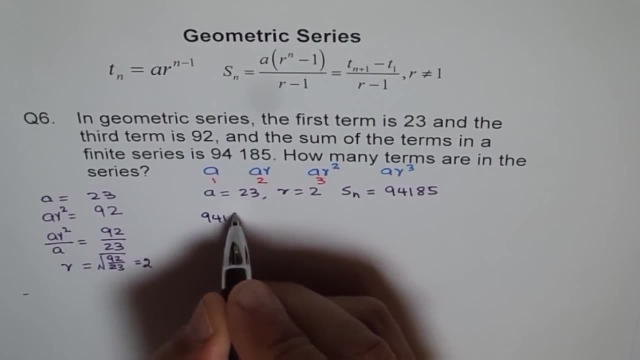 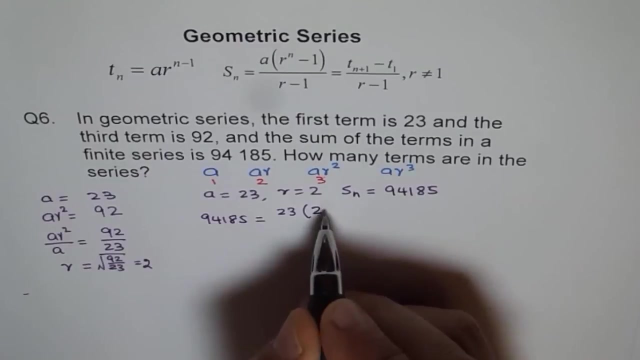 we'll use this formula: s of n equals to this. Using this formula here, we get 94,. 185 equals to a is 23,. so we get 23 times r is 2,. 2 to the power of n minus 1, divided by 2 minus. 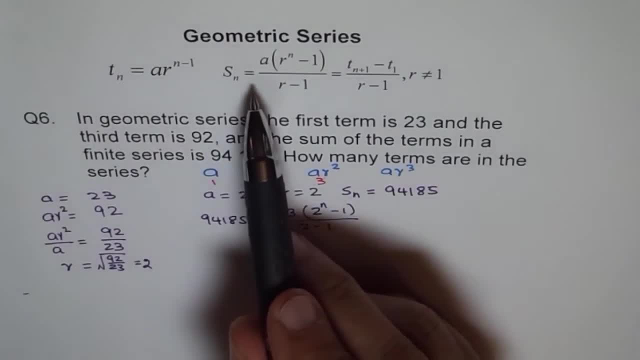 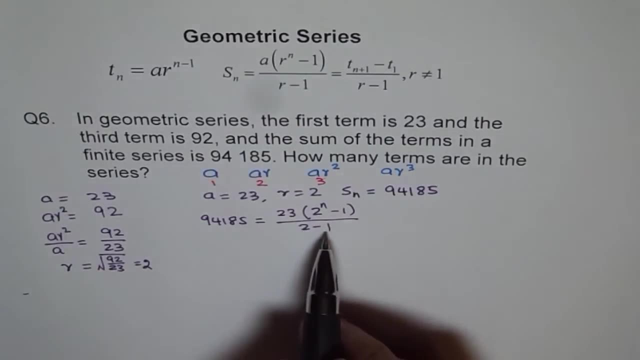 1. Correct, So we use this formula: s of n equals to a times r, to the power of n minus 1, divided by r minus 1.. Now 2 minus 1 is 1, so we are left with this divided by 23,. so we get. 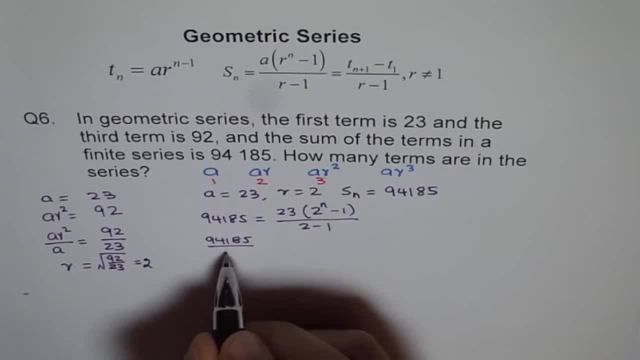 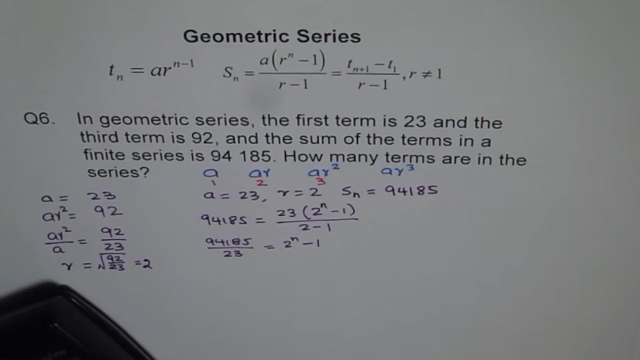 94, 185 divided by 23 equals to 2, to the power of n minus 1, correct, Let's do that: 94, 185, 94, 1, 9, 4.. So 1, 8, 5, divided by 23 is equal to 4, 0, 9, 5.. So here we get 4, 0, 9, 5, 4, 0, 9, 5.. 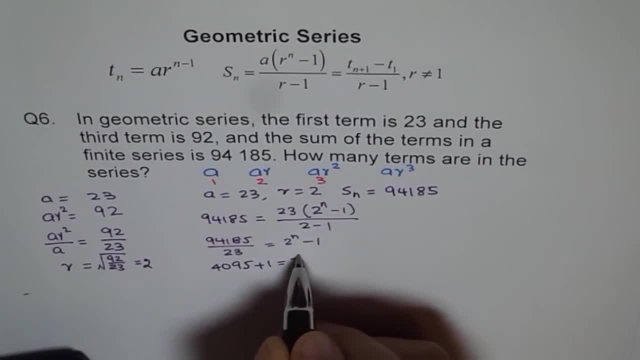 I'll bring 1 this side. so plus 1 equals to 2 to the power of n. Now, from here we can find what n is. So what to the power of 2? to the power of what is 49?? 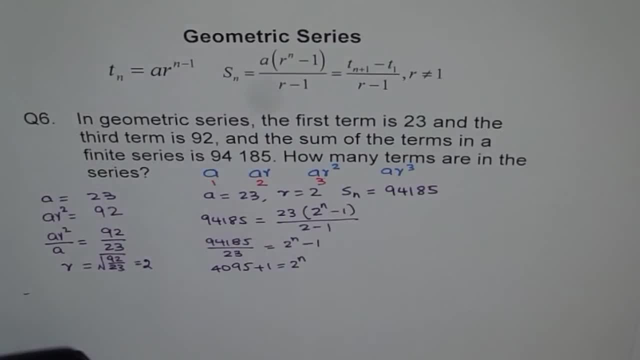 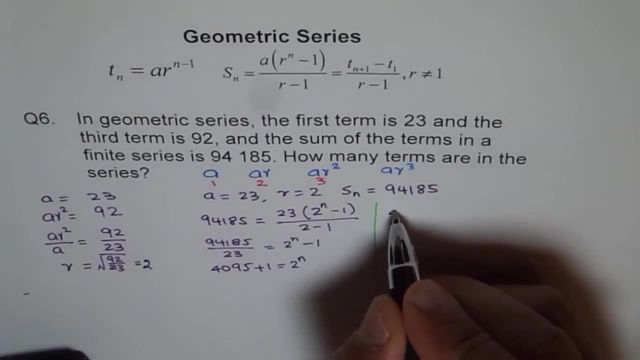 496.. That is what we need to find now, right? So there are a couple of ways to do it. Let me write this first. here We have: 496 equals to 2 to the power of n, We know, 2 to the power. 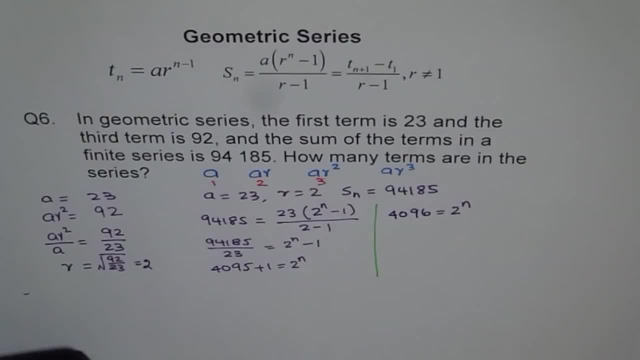 of 10 is 1024, so 2 to the power of 11 will be 2 times 1024,, which is 2048, and 2 times 12 will be 496.. So that is how we get n equals to 12.. 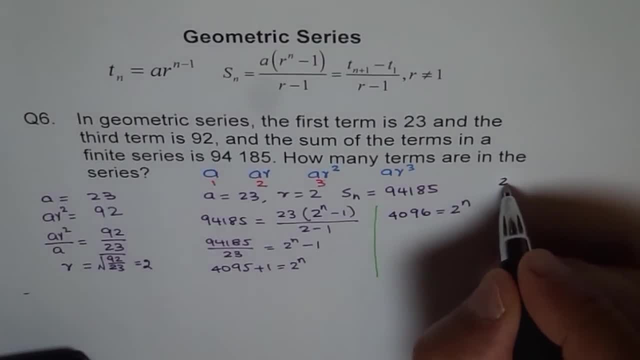 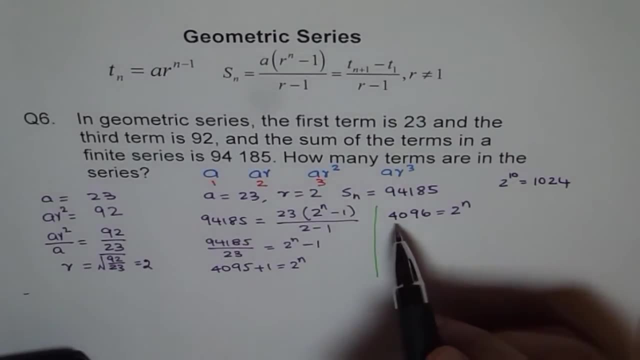 Right, Remember all this. What is 2 to the power of 10 equals to 1024, correct? Remember that If you multiply once by 2, you get 11,, which is 2048, and then again by 2,. that means: 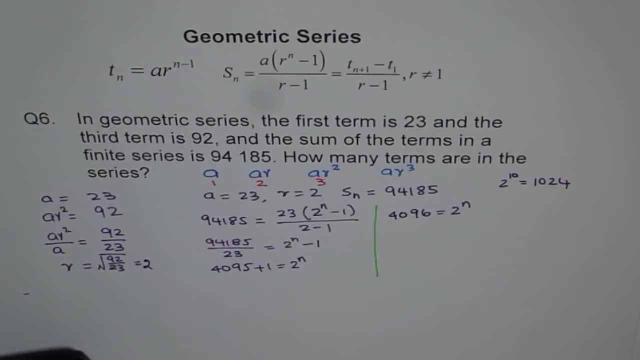 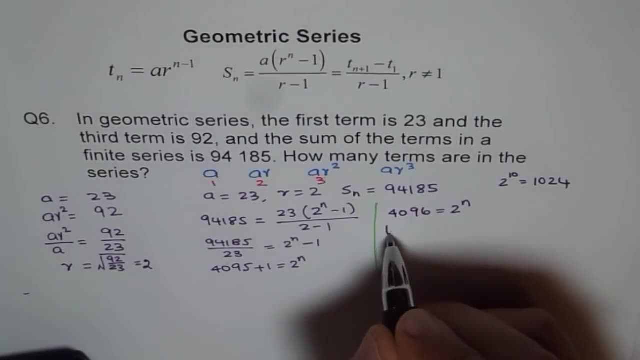 2 to the power of 12, we get 4096.. The other way to solve such kind of equations is to take log both sides, right? If we take log both sides, we get log of 4096 equals to 2. 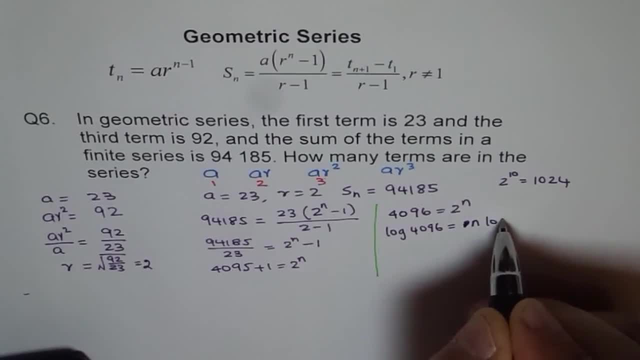 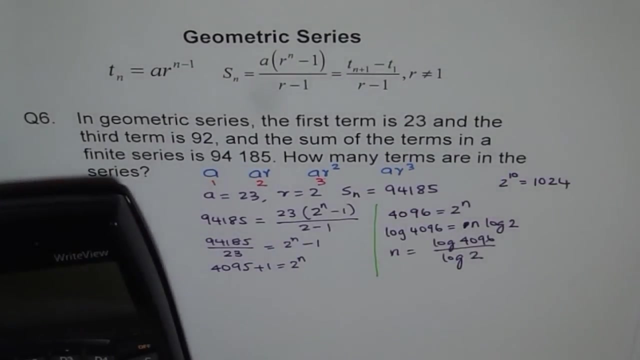 times 1024. Right, Sorry, n times log of 2, right? And then we can find n from here. n is equals to log of 4096 divided by log of 2.. So let's try the second method: Log, right. So it says. 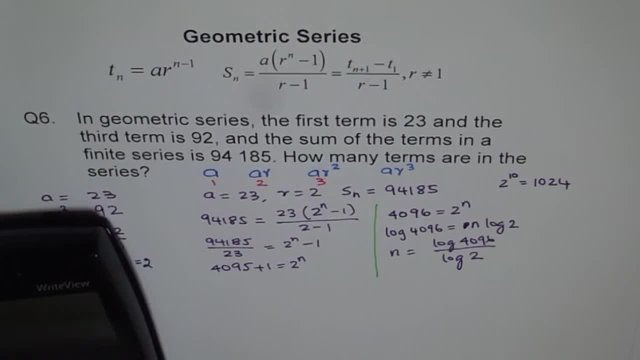 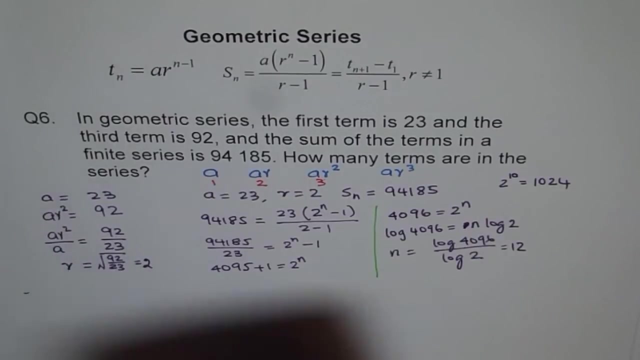 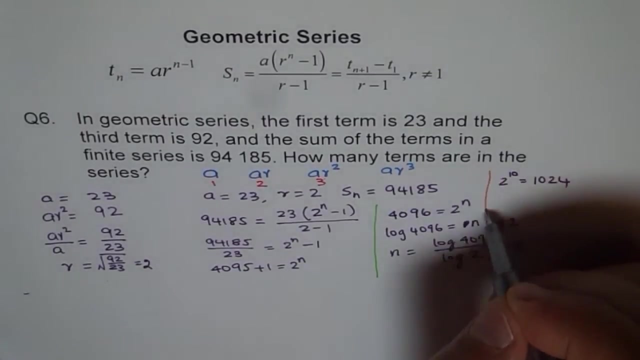 log of 4096 divided by log of 2.. n equals to 12.. So we get equals to 12 here, right? So n equals to 12.. So it's the same. We got 2 to the power of 10.. We could have also calculated like this: 2 to the power. 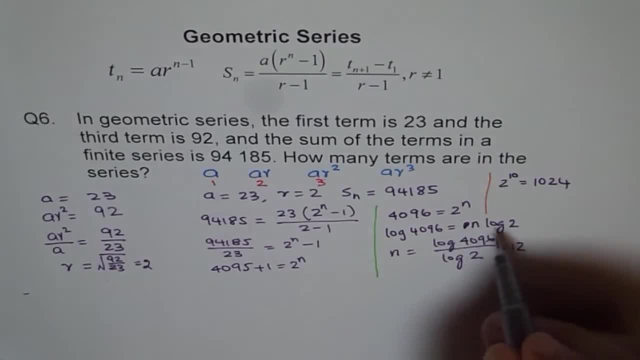 of what is 4096?? Sometimes, if log is not, that calculator is not there with you. you can try. like this, right? So we know: 2 to the power of 10 is this. So 2 to the power of 11 will be times 2,, which is 2048.. And 2 to the power of 12..